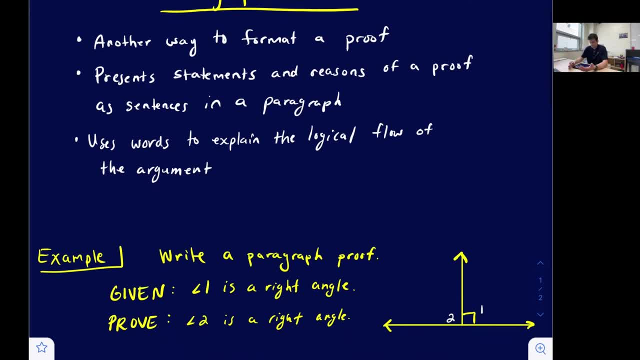 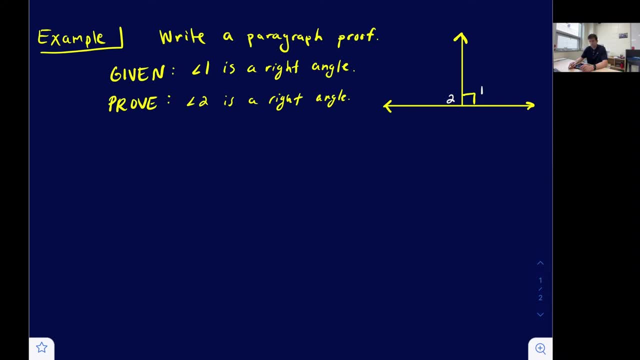 We're going to use words to explain the logical flow of the argument. Okay, so we're going to look at an example and they just tell us to write a paragraph proof. So if you're struggling with a paragraph proof or even a flowchart proof, maybe you like two column proofs. but the question 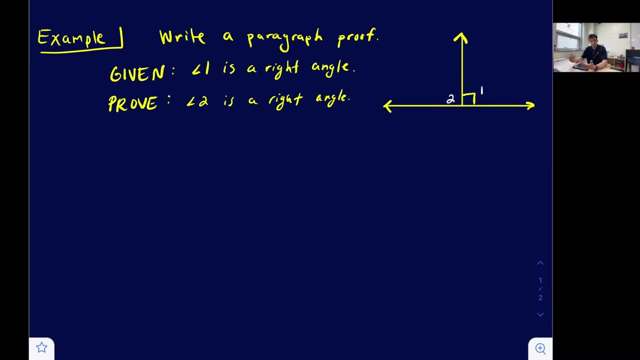 calls for a paragraph proof. You could always write the two column proof and then just transfer that as sentences in a paragraph. So we'll go ahead and look at our diagram. here We have two lines. They form perpendicular lines. here We can see we have a right angle box. 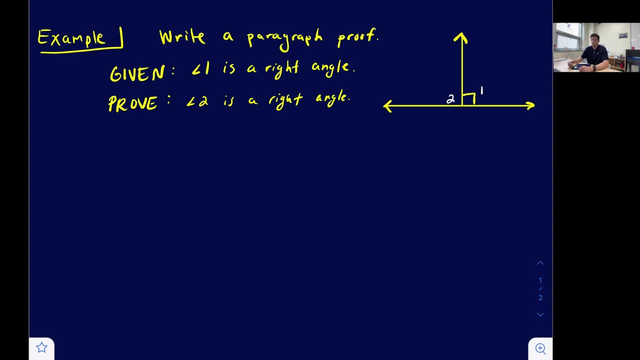 at angle one which tells us the given statement. angle one is a right angle, So we're going to start with that in our paragraph. Angle one is a right angle, Okay, and that's going to tell us something about that angle right, And that means its measure. 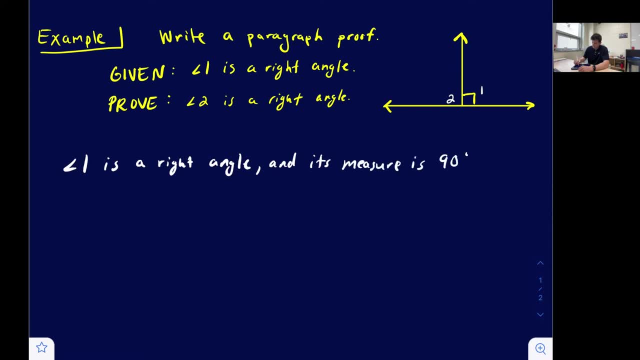 is 90 degrees. Okay, by what definition? By the definition of a right angle. Okay, so basically, we've used our given statement. Okay, All, right. now we look at angle one and angle two. Angle one and angle two. they actually I'm not going to say they- angle one and angle. 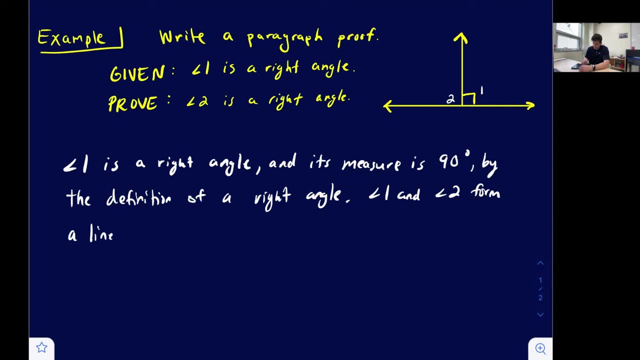 two form what's called a linear pair. Okay, so we can say, by the linear pair, postulate the measure- I'm going to write it down here: the measure of angle one plus the measure of angle two must equal 180 degrees. Okay, So these angles, 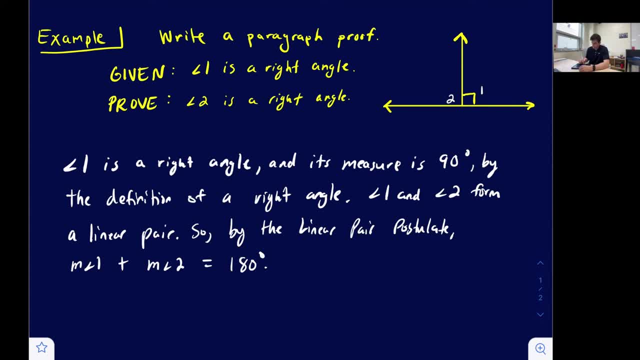 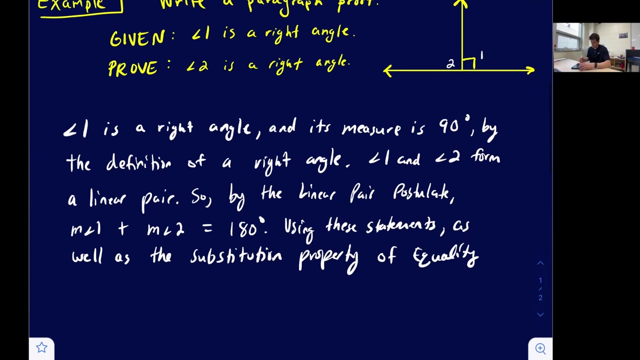 are supplementary right. So now we can use these statements. So we can say, using these statements as well as the substitution property of equality, we could now substitute in 90 degrees for the measure of angle 1.. So, using these statements as well as the substitution property of equality, 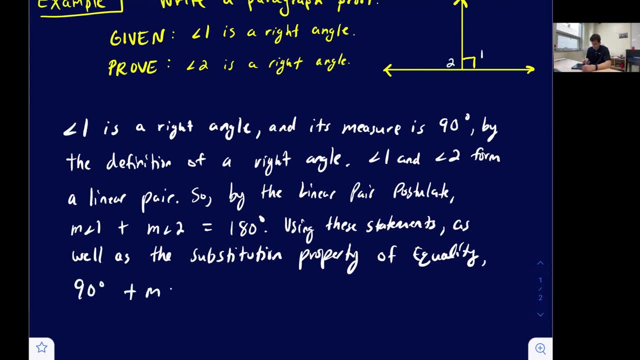 we could say: 90 degrees plus the measure of angle 2 equals 180 degrees, right? So algebraically you're looking at that and going: okay, we could subtract 90 from both sides. That's exactly what we can do.